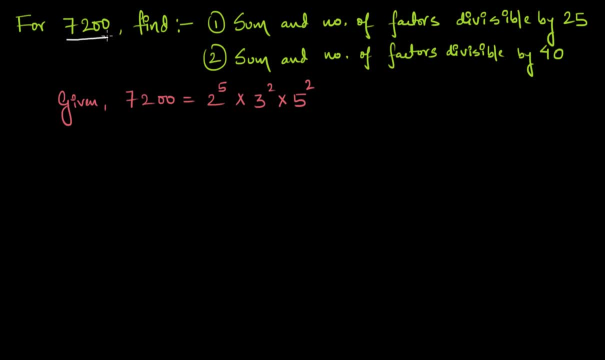 For 7200, find sum and number of factors divisible by 25 and sum and number of factors divisible by 40. So before solving it, let us first of all write down sum of all the factors of 7200.. So sum of all the factors of 7200 will be equal to. let us start with the minimum possible power. 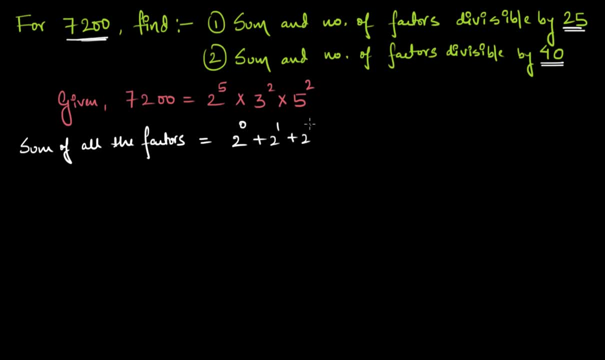 of 2 to the power 0 plus 2 to the power 1 plus 2 square, and we will take it to the maximum power of 2 available here, that is, 2 to the power 5.. This thing multiplied by 3 to the power 0 plus. 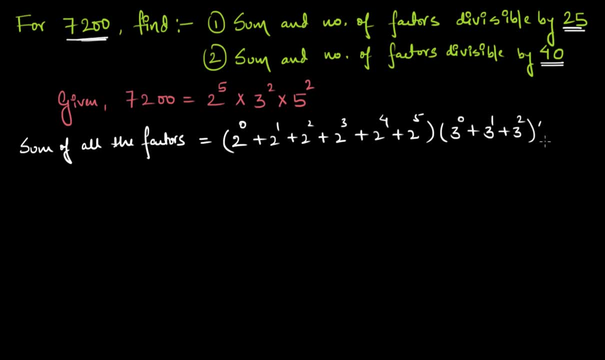 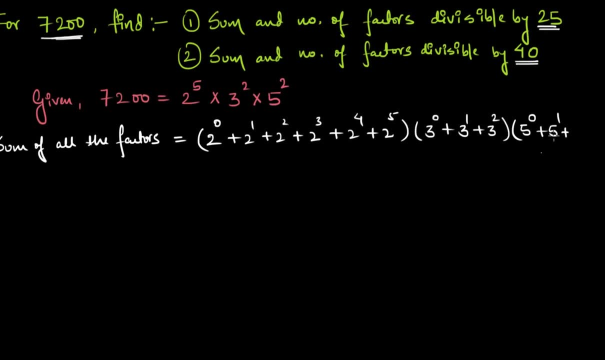 3 to the power 1 plus 3 square and 5 to the power 0 plus 3 to the power 1 plus 3 square, 0 plus 5 to the power 1 plus- let me shift the screen a bit- plus 5 square. So this is sum of: 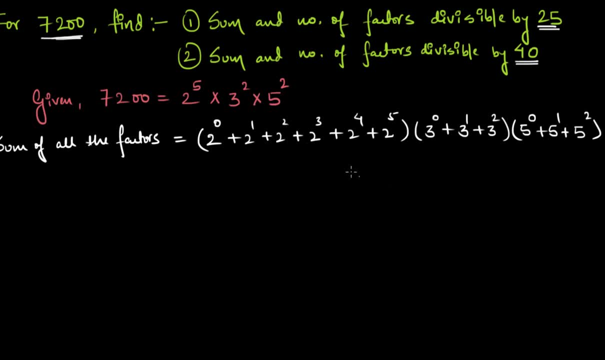 all the factors. When I multiply them, each term will represent one of the factors of 7200, and all this thing, multiplied together, will give me sum of all the factors of 7200.. But now we are asked to find only those factors, sum of only those factors, which are divisible by: 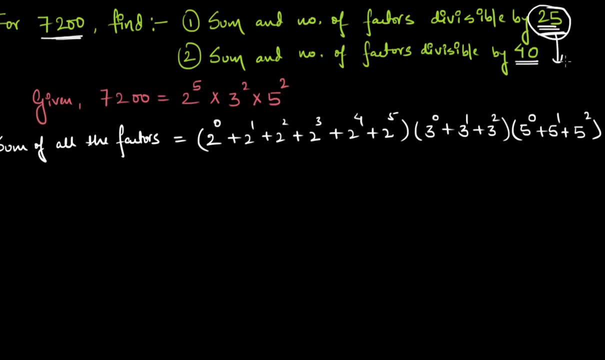 25.. Now, how can I get a 25? If I will have at least two 5s, 5 times 5.. If I will have two 5s, I can get a 25.. So all the terms which will have 5 square, 5 square in it and sum of all such terms. 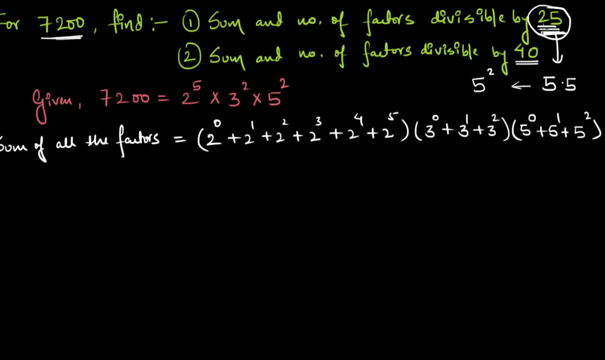 will give me all those factors of 7200 which are divisible by 25.. But in this expression, how can I be assured that all the terms contain a 5 square? So what I will do, I will just remove the remaining, This 5 to the power 0, it makes no sense because I need at least a 5 square. 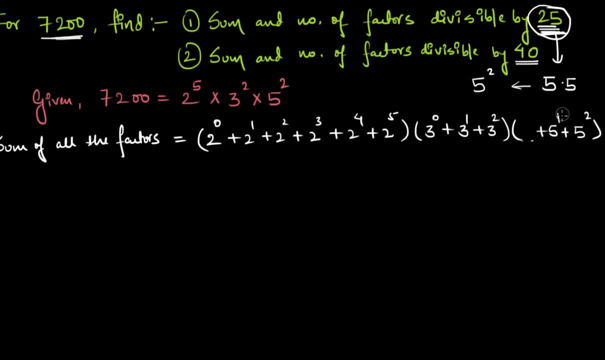 So I will just remove this 5 to the power 0 and 5 to the power 1, because for 25, I need at least two 5s, So even this won't count. So I will just have a 5 square, 5 square. Now when I multiply. 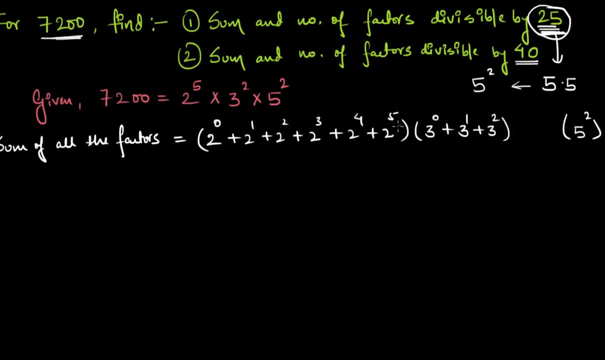 all of them, all the terms will have 5 square in it for sure, And the sum will give me the sum of all the factors that are divisible by 25.. This thing we can calculate easily. I just wanted to show you how we can come to the conclusion that, how we can find the sum of all the factors that 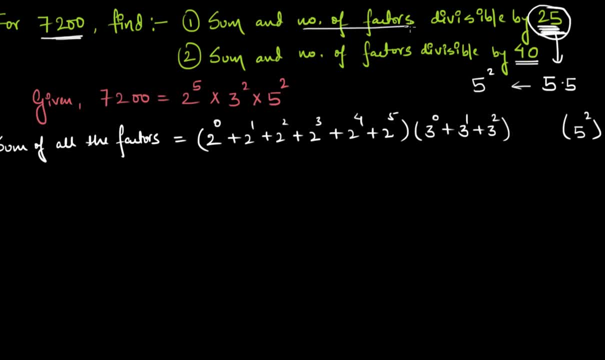 are divisible by 25.. Secondly, we are asked to find the number of such factors. Now, all the terms that we will have here, all the total number of terms present in this expression, will represent. each of the terms will represent an individual factor of 7200, which is divisible. 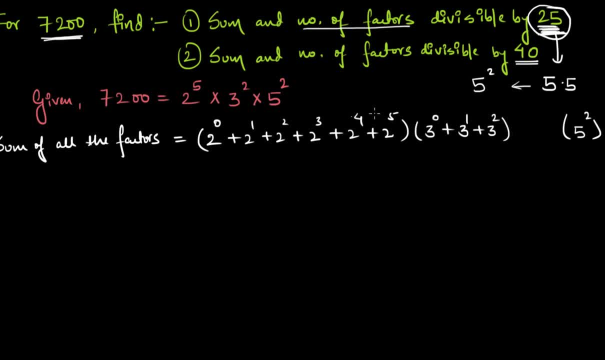 by 25.. So what we can do here? we can just find the total number of terms present in this expression. So for each term to be built from this expression, I have to take, I have to take at least one term from this part. So here I have total six terms. 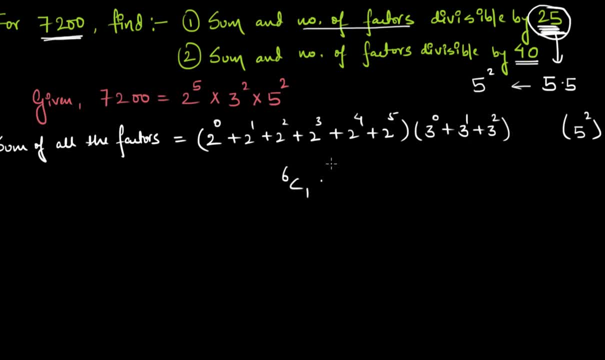 So I'll just pick one from this, pick any one from this. three say one, and we have to take this. we have to always consider this. So just one possibility. So total number of terms present: six times three times one, that is 18.. So there will be 18 such factors. 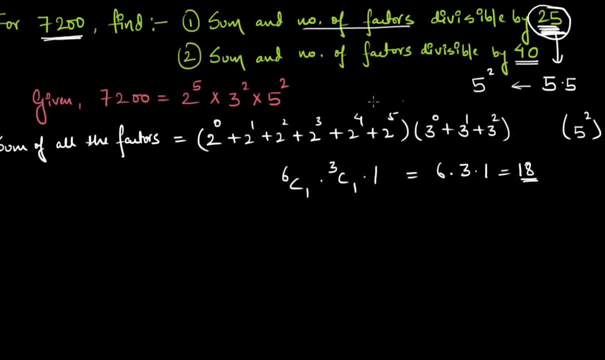 which will be divisible by 25.. And we know how can we find the sum of those factors: by just finding the value of this thing and this thing and this thing and multiplying them all together. Now, what can be said about 40?? Now for 40,, for 40, I can write it as four times 10,. 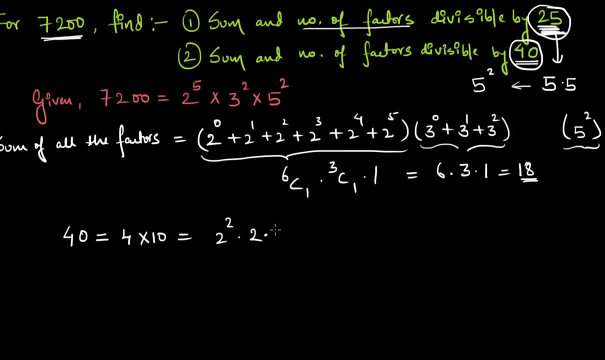 which is equal to two square times two to two multiplied by five, which is equal to two to the power five- sorry, Not two to the power of five. two to the power three times five. This will give me 40, because this is the prime factorization of 48, fives of 40. So in order to get 40, I need at least three. 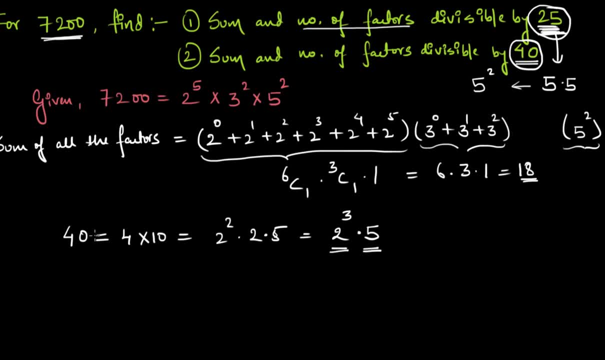 twos and one five, then only I can get a factor which is a multiple of 40.. So let me write the initial total number of factors: sum of all the factors which will be equal to five, to the power zero plus five, to the power one plus five square, This will represent the total number of fact. 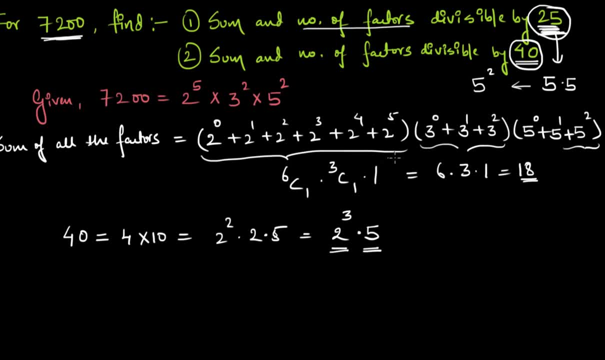 sum of all the factors, which will be equal to five to the power zero plus five to the power one plus five. sum of total number of factors of 7,200.. Now I want that all the terms should contain three twos, at least three twos and one five, because if any term will have two to the